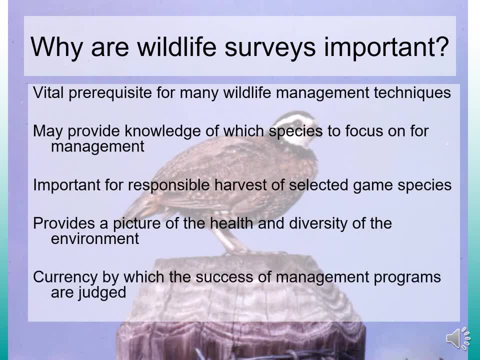 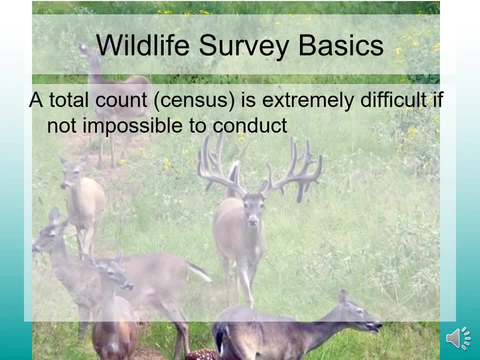 of the health and diversity of the environment. They're also the currency by which the success of your management programs are judged. So a little bit about wildlife survey basics. A total count, or census, is extremely difficult, if not impossible, to conduct for most wildlife. 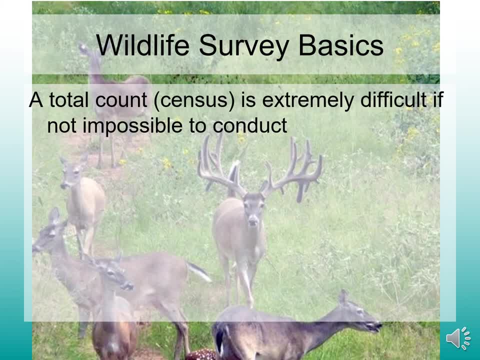 species. Things like white-tailed deer or grassland birds or things like that will be moving around quite a bit and we won't be able to tell every total individual, so we have to use surveys to get an idea of the population, but we'll never know the exact number of animals. 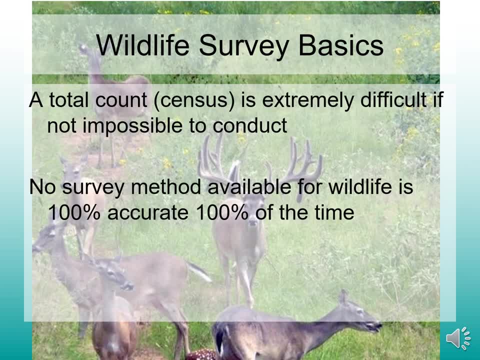 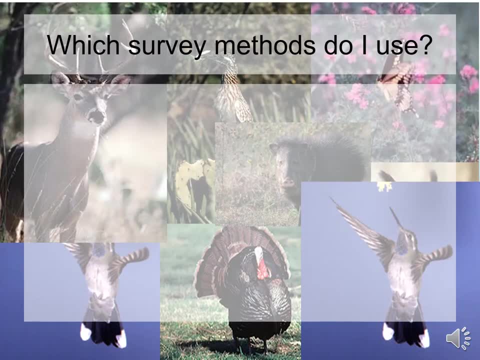 Furthermore, no survey method available for wildlife is 100% accurate, 100% of the time. So it is best to conduct multiple surveys and compare the results. So which survey methods do I use? Well, first, what wildlife species are you interested in? Secondly, how much time do you have? Third, how much area are you? 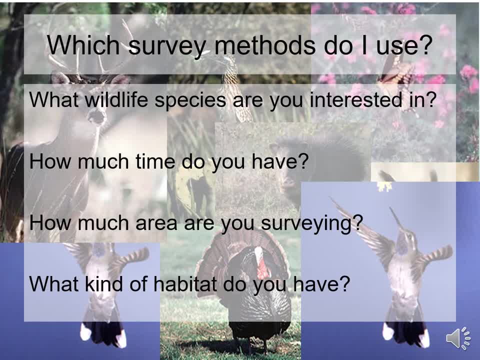 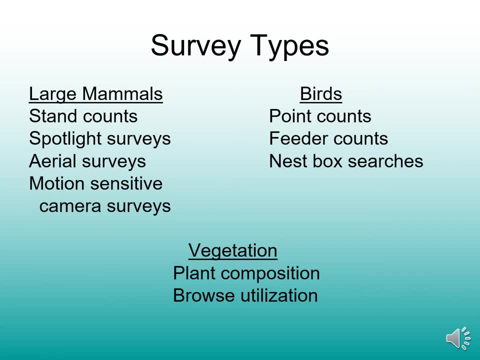 surveying And finally, what kind of habitat do you have? There are several different survey types that are available and we could, by working with your biologist, depending on what you're interested in, we could help you develop a survey that would work for you. But right now we'll go. 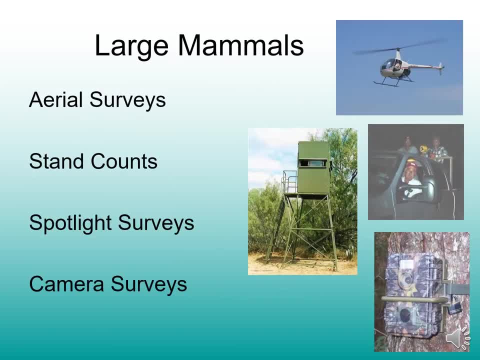 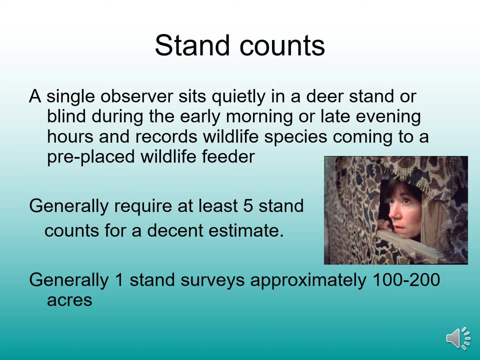 over some of the primary survey method types that people use For large mammals. the primary survey methods include aerial surveys with helicopters, stand count surveys, spotlight surveys or game camera surveys- Stand counts kind of how they sound. you basically sit in a deer, blind, with a. 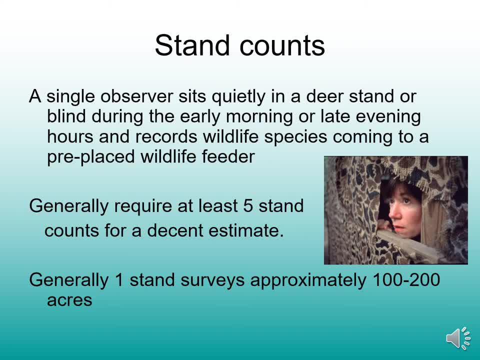 pre-placed wildlife feeder and you count the wildlife species you're interested in. So you're interested in that, come out to that feeder. Generally it requires at least five stand counts for a decent estimate And generally one stand can survey approximately 100 to 200 acres. 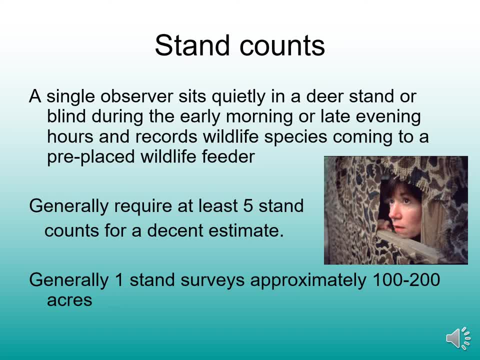 Ideally it would be best, if you have multiple stands, to put people in every single stand and count all the deer you're seeing, or pigs, or javelin or whatever species you're interested in. to get a good survey estimate, Spotlight surveys require a pickup truck, a driver and two observers. 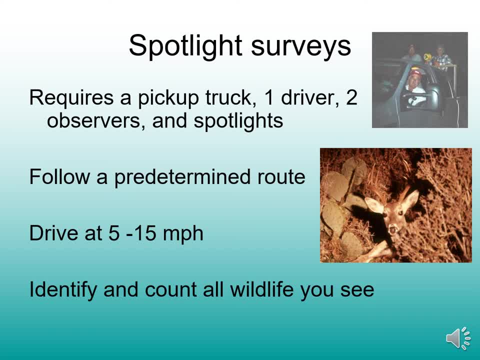 with spotlights, You develop a predetermined route through the different habitat types, Drive at about 5 to 15 miles an hour and identify and count all the different nocturnal wildlife that you see. Also, it's probably a good idea to reach out to your local game ward and let them know when. 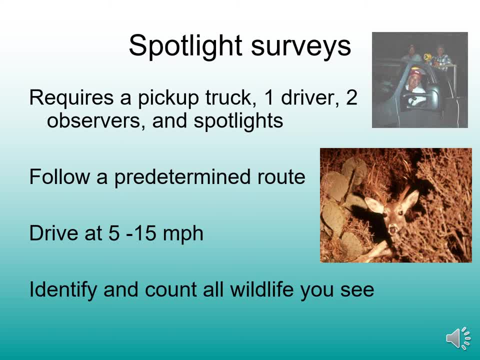 you're going to be doing a spotlight survey so that they don't come up on you and try to wonder what you might be doing while shining a spotlight at night. That way they can be available for other things that might happen that night besides just you. Another one are camera surveys- Camera. 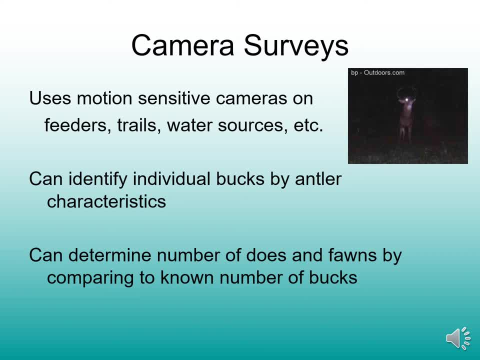 surveys, use motion sensing cameras on feeders, trails, water sources etc. And for whitetail deer. they can be used to identify, monitor and monitor wildlife. In some cases they can be applied by adding a GPS. A fine-tuned animal scout is a good way to. 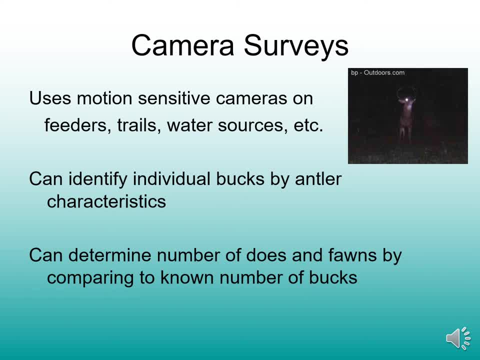 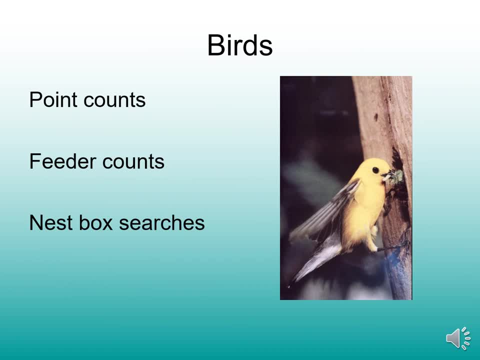 identify individual bucks by any of their characteristics and determine an estimate of the number of bucks you have on the property. Then you can compare that to the total number of doe and fawn pictures to get a full population estimate For birds. several different survey. 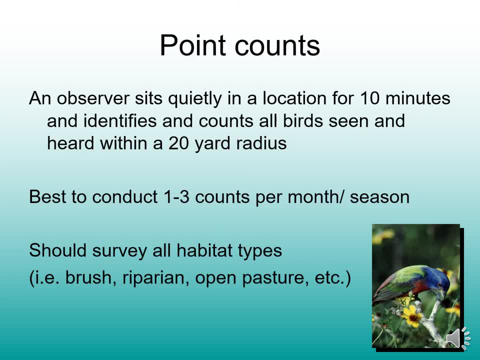 methods can work. One of those is point counts. The point count- an observer sits quietly in a location for up to 10 minutes, identifies and counts all birds seen and heard within a specific radius. It can be 20 yards or it can be even more than that, depending on the species you're interested in. It's best to conduct one to three counts per ml per month to see if there are plenty of birds seen from a certain range. 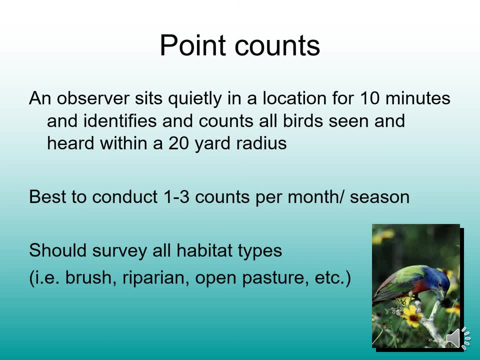 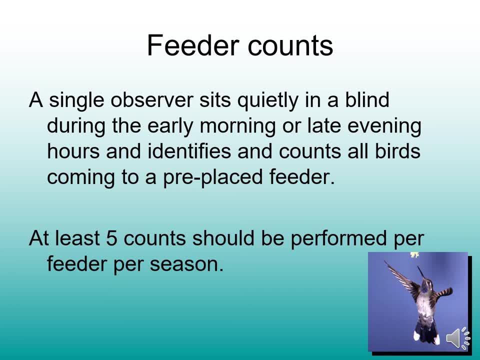 month or season, and you should survey all the different habitat types on your property. Feeder counts are very similar to the stand counts in that you sit at a predetermined location with a feeder within sight and you count and identify the different species that are using that feeder. 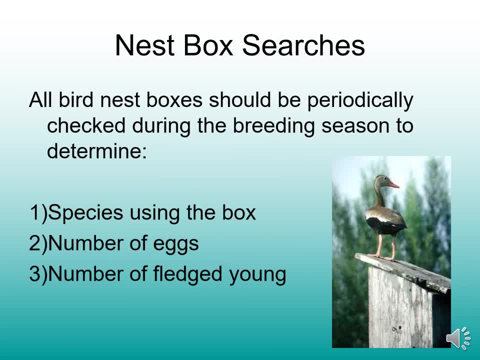 At least five counts should be performed per feeder per season. Nest box searches, as the name implies, is when you put up these supplemental shelter nest boxes, evaluating those annually to see which ones are used and what species are using them. I generally don't recommend counting the eggs or the young by disturbing them, but maybe 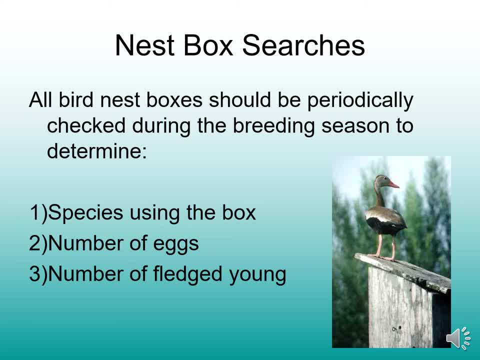 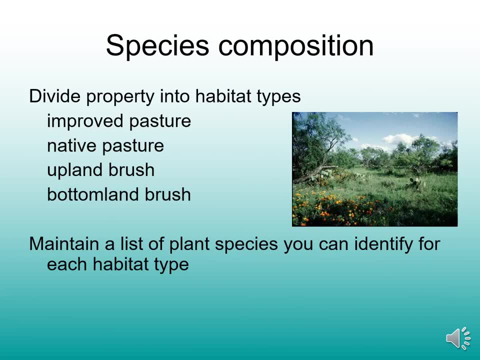 just seeing which ones are used and which ones aren't and identifying the species would probably be the best thing to do. You can also do vegetation surveys. One thing you can do is identify all the different plants that are on the property and maintain a list of that and look at the different habitat types. 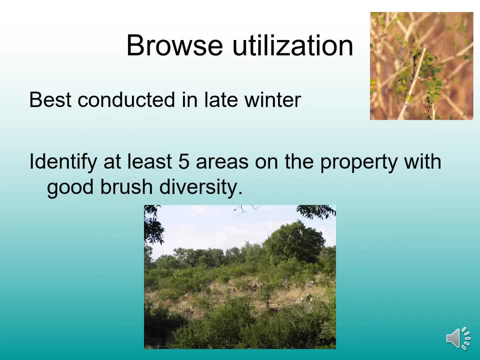 You can also use a map. Just use browse utilization. Look at how the impact of species like white-tailed deer have on the habitat that they're using. It's best to identify at least five areas on the property with good brush diversity to conduct this browse survey.